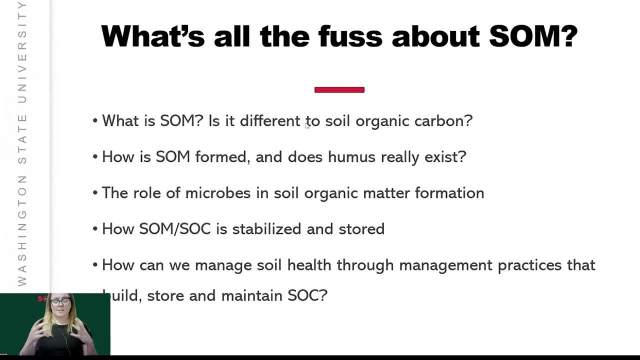 organic matter is one of those things that we all know that it's really important and we need to have it in our soils. but it's kind of like when the doctor tells us to eat more vegetables, We say okay, okay, and we do it, but we don't really always know why. So what is soil organic? 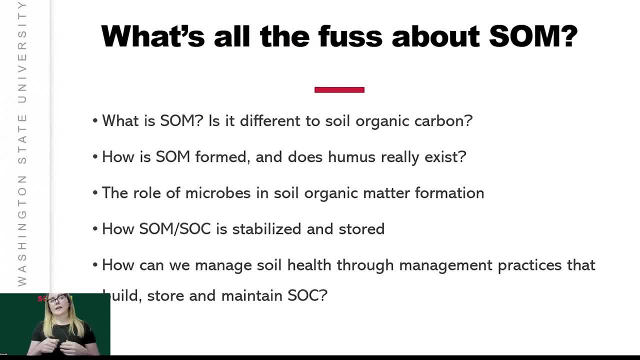 matter, and is it different to soil? organic carbon? We're going to look at, as I said, how it's formed and also, does humus really exist? Humus and humic substances have been a bit of a buzz to the agronomic community for a very long time, so we're going to talk a little bit about. 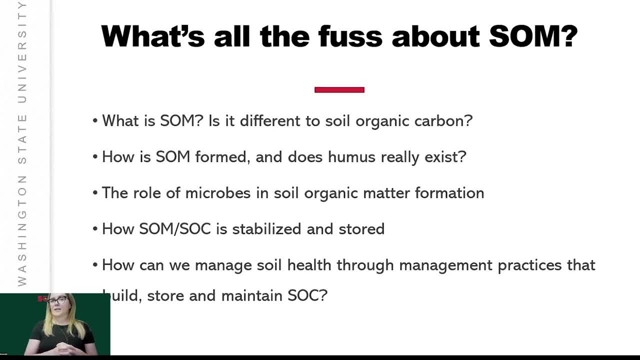 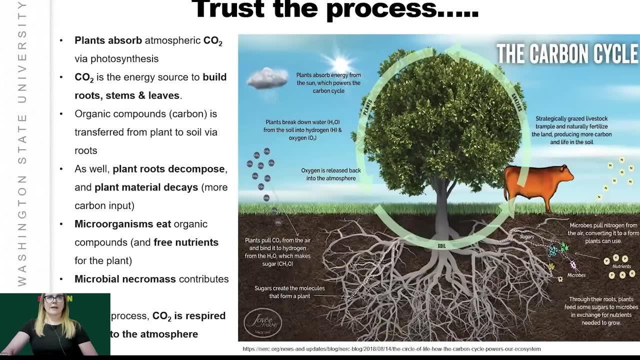 that And the role of microbes in soil organic matter formation. Randy has touched on a little bit of that and how SOM and SOC is stabilised and soared in soil And also how can we manage our soils better to build, store and maintain soil organic carbon. 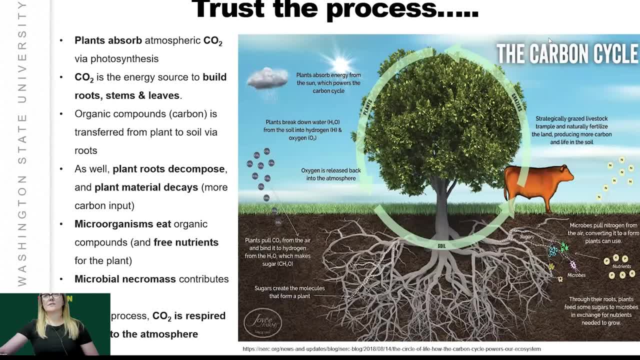 over time. I'm just going to see if I can move this little thing there. There we go, All right. So for those of us who don't know a heck of a lot about how soil organic matter starts: basically, Without plants we're not getting that continuous carbon into soil, So plants absorb the atmospheric. 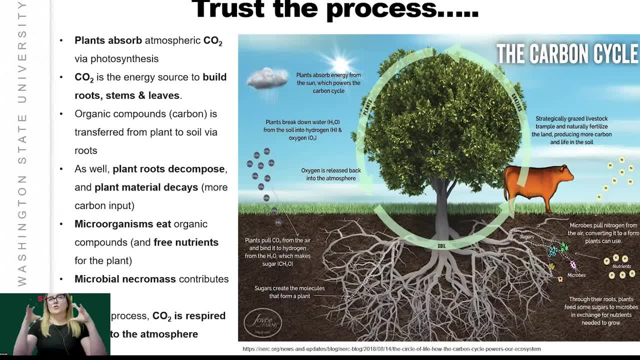 CO2 and they use that atmospheric CO2 to build their structures- leaves, stems, roots- but also they push organic compounds, primarily carbon, down through those root structures and into the soil As well. those plant roots decompose organic matter that is on the surface of the soil also. 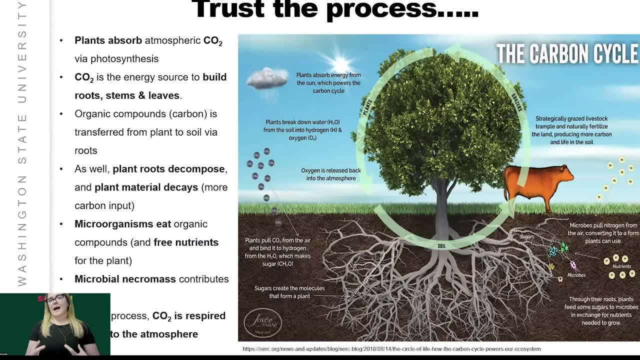 decomposes And as it decays we get more carbon input into the soil. And then the role of microorganisms becomes a little more important, where they're sort of eating up all of those organic compounds. And in the process of eating up those organic compounds they're freeing nutrients for the plant. 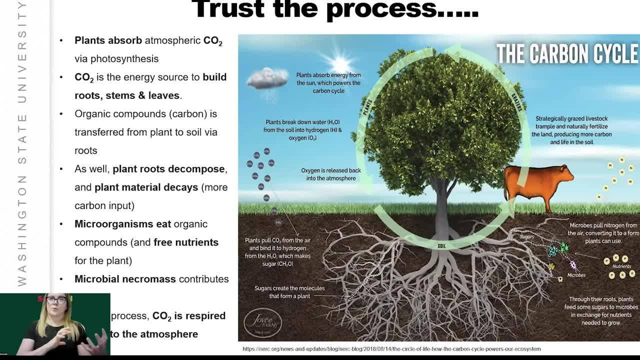 So this is very much a symbiotic relationship between the plant and the soil microbes. Microbial necromass, which Randy also discussed before, contributes a lot to the organic matter And we're really starting to understand how important that relationship is. But it's important to note that at each level of this process CO2 is respired back into the atmosphere from the soil surface. 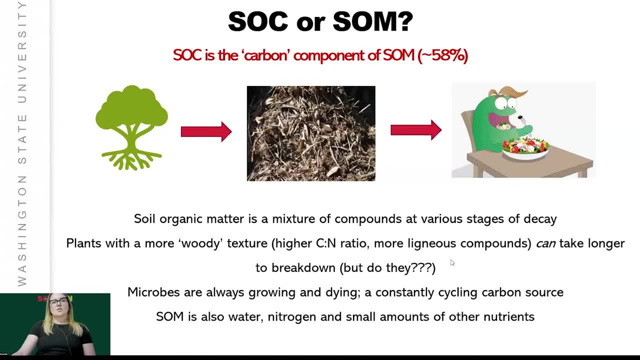 So SOC or SOM, they are sort of essentially the same thing. Soil organic carbon is the carbon component of soil organic matter. It makes up about 58%. It also has water, nitrogen and other small amounts of nutrients. But soil organic matter itself is a mixture of compounds at various stages of decay. 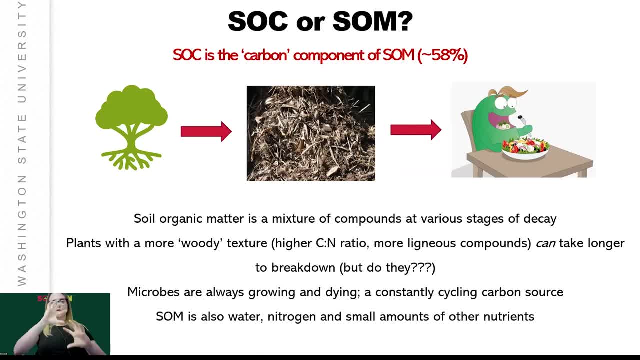 So we're looking at something that is really a mixture of all different things, You know, plant residues, animal residues, things like lignin compounds, a little bit more woody textured plants And microbes are always growing and dying, which again contributes to decay. 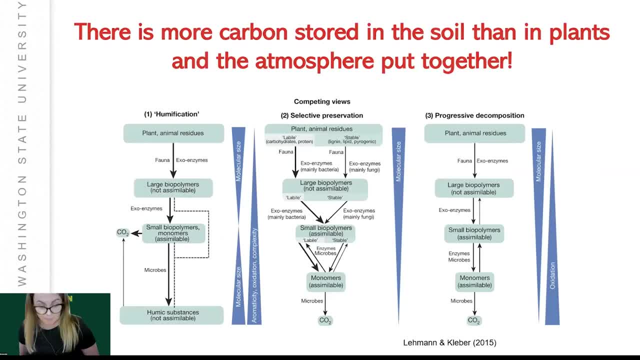 But scientists, still to this day we like to argue about how soil organic matter is formed and how it stays there. So there have been sort of has been sort of a progression of competing views over time, starting with one of the kind of older ideas about soil organic matter formation. 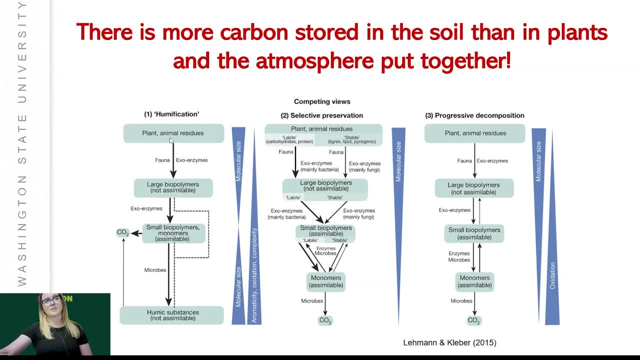 And that is the human body And that is the humification concept. So the idea is that we have these plant and animal residues that are broken down in soil by exoenzymes that are secreted mostly by microbial communities and soil fauna, And then they get broken down into these larger biopolymers. 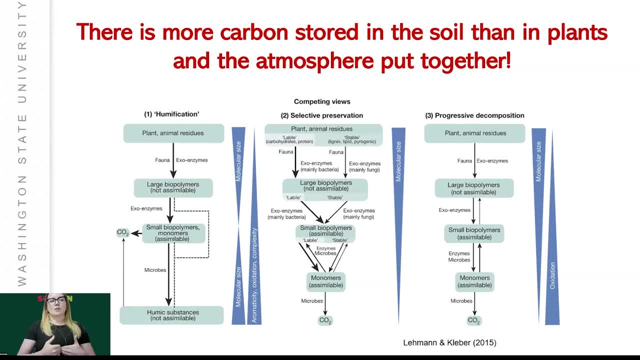 And some of these biopolymers were said to be non-assimilable, as in they can't be taken up and kept by microbes. But there's also a part of this process where these large biopolymers were being essentially stabilized through these abiotic processes. 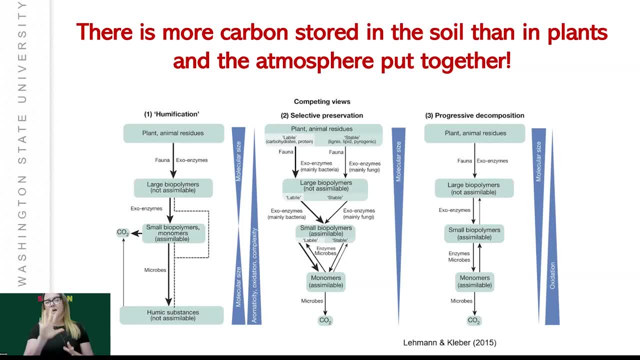 So non biological processes that weren't really very well understood And those became called humic substances And then through that progression of more and more exoenzyme decay And again these microbes that just kind of got shoved in down the bottom there without really understanding. 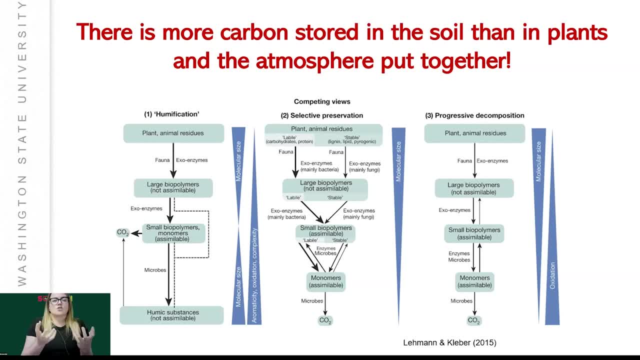 what their role was. We end up with this humus, as it was called. Unfortunately, there was a little bit of methodological issue with the way that humic substances were being characterized. They used some very kind of forced extraction methods that essentially meant that we were 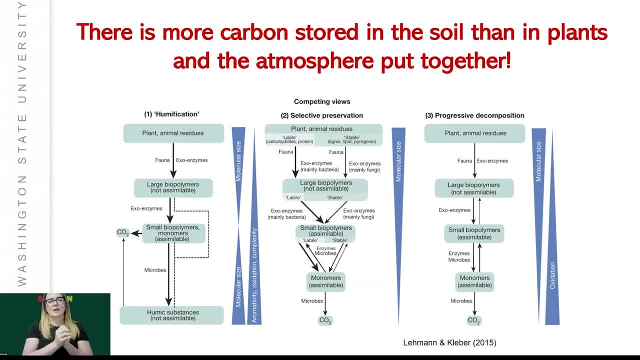 ending up in soil with these humic substances that were not necessarily products of soil organic matter degradation, but were more operationally defined. Then the second concept was that of selective preservation. Again, you start with these plant and animal residues, and then there 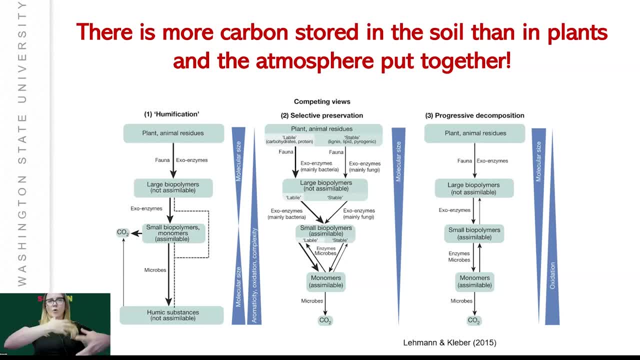 was this idea that there was more labile, so more easily consumable, compounds, and then these more stable compounds, compounds in soil, organic matter. As I said before, those might include things that have a higher carbon to nitrogen ratio or contain lignin. Again, there was this exoenzyme breakdown. 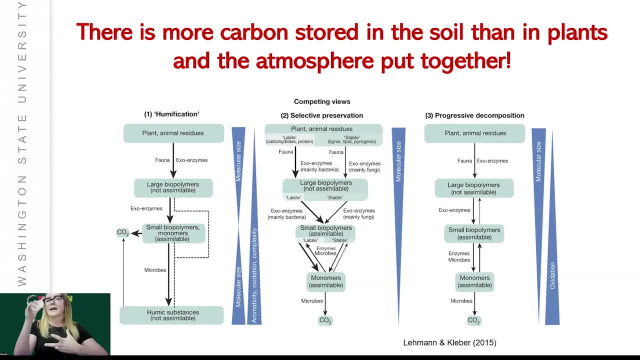 mainly through bacteria for those more labile compounds, and then fungi were kind of attributed as the ones that broke down the more stable compounds. Again, we go from larger to smaller biopolymers, down to monomers, and then again microbial decay and then CO2 goes back into the 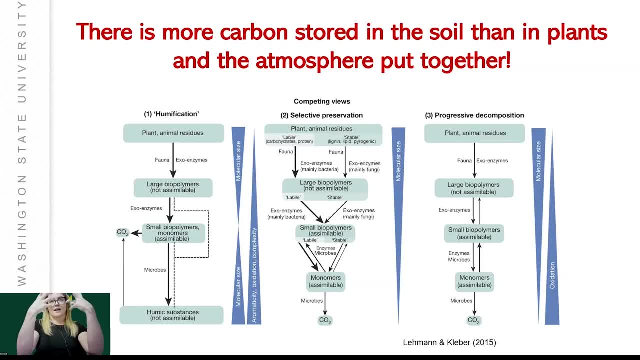 atmosphere. So essentially there was this idea that there was almost like, as the microbes were eating, they were choosing what they were able to take and what they couldn't. And then the next one, progressive decomposition, sort of similar to selective preservation but more kind of 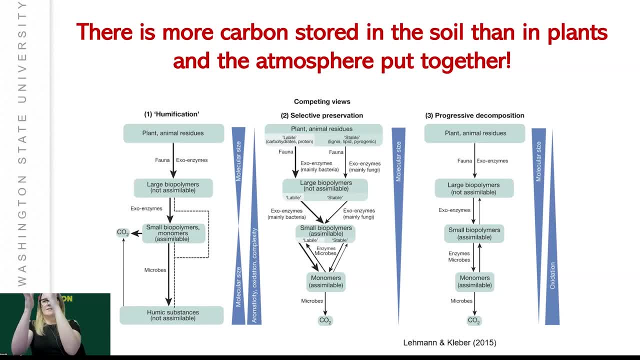 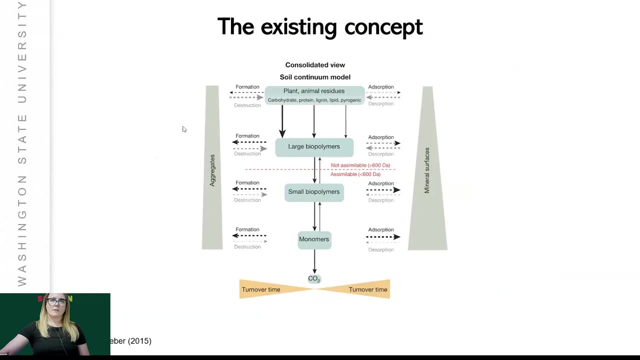 also says that, as these molecular size decreases through the process of decomposition, that they're more highly oxidized compounds that we are left over with. And then we have come finally to a more consolidated view over time, And this is by work from Lehman and Cleaver in 2015.. So it's a very, very good example of a 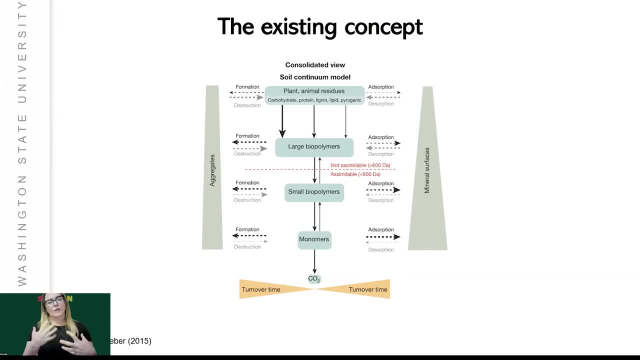 model that we can kind of continuously work with today. It sort of consolidates a little bit of that progressive degradation and selective selection model, But it also focuses on the role that soil minerals and aggregation play in stabilizing soil organic matter and soil organic carbon. So we again, we have those residues, we have those residues, we have those residues, we. 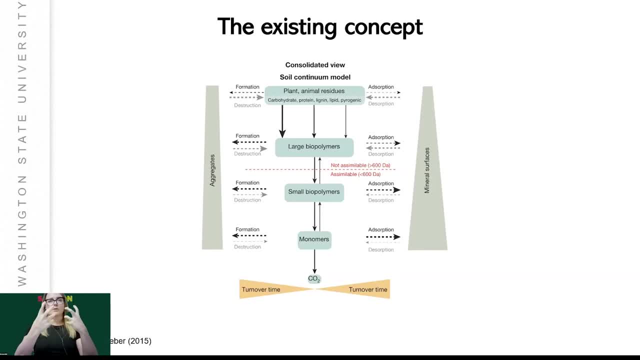 that are broken down by microbial processes. but in the process of those breakdowns they will sorb or attach onto mineral surfaces and also they can form into aggregate structures, where the soil organic matter belongs onto soil particles, and then particles come together and at the same time all of these processes are again reversible. so it's not that the soil 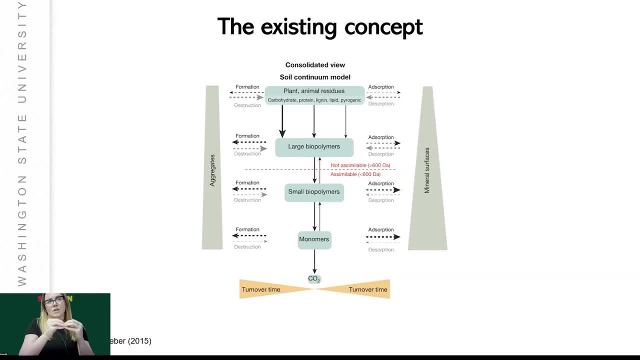 organic matter just sorbs onto minerals, or that the aggregates are just formed, but that they can also desorb from mineral surfaces and also be destroyed in aggregates. So essentially the whole idea is that the more aggregated soils are with the soil organic matter, the more mineral. 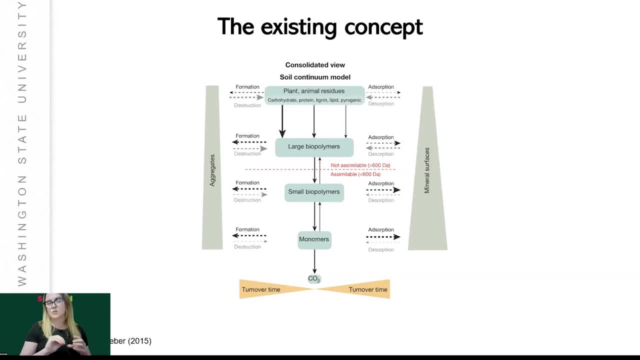 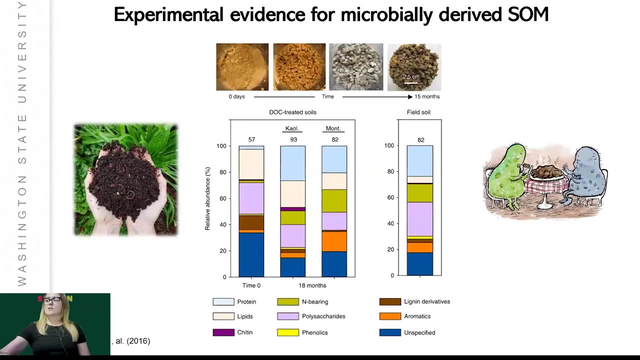 associations. so Randy talked about malm, so that is primarily what I'm talking about. with mineral association You're getting a longer turnover time where you have those aggregate structures and mineral sorption. so this is a little bit of a really exciting experimental evidence for microbially. 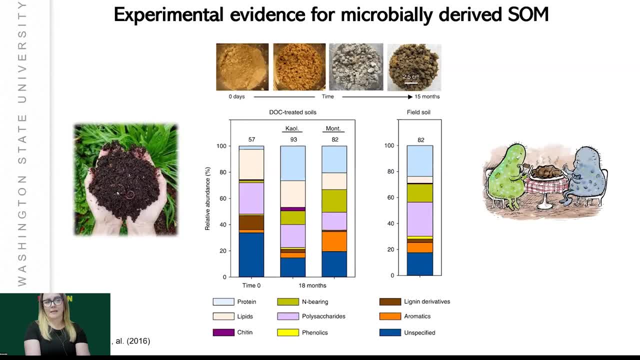 derived soil organic matter. This is some work by Kallenbach et al in 2016.. Essentially, what these guys did was they just took the basal mineral matrix of soil. They essentially took two different types of clay minerals- kaolinite and montmorillonite- and they just put them into incubation containers and they added some. 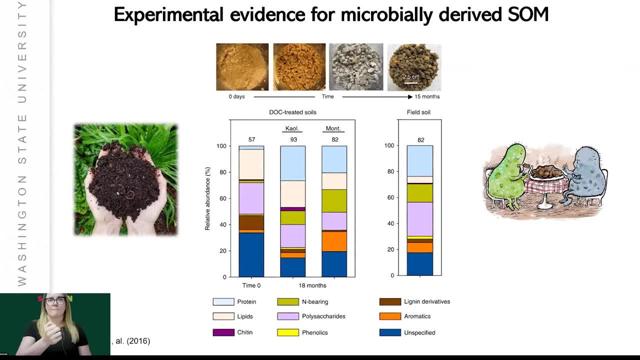 organic acids and dissolved organic carbon to them over a period, continuously, over a period of 15 months. And so you can see, here there is this kind of. this is the soil at time, I guess you can. this would be, I guess, a little bit more like dirt at this point, as people might want to say, but it was more of a mineral matrix that was pretty much kind of dominated by, by lipids. We have like some polysaccharide here, some lignans derivatives. 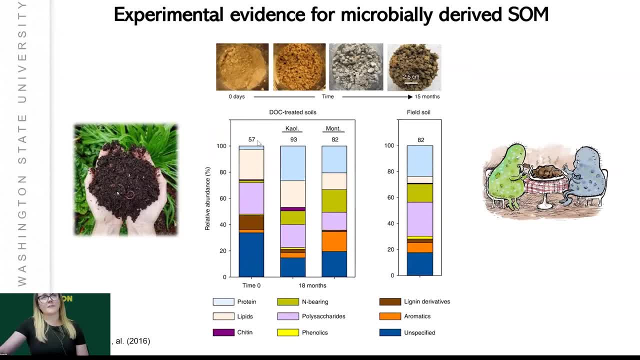 And a lot of unspecified compounds, but just a total of 57 compounds. What I should also say, too, is that, in addition to the organic acids and carbon that they put into these soils, they also added a little bit of a microbial inoculant. 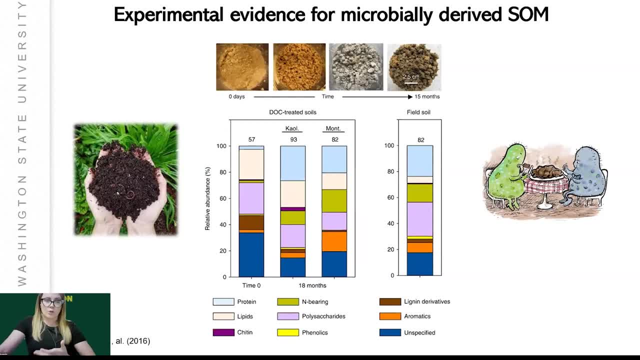 so that because these soils didn't have the microbial community before, that would allow that microbial community to start doing things with the compounds, Essentially over time. in a time of 15 months these microbes turned this dirt into soil. We had up to 15 months in the different soils. 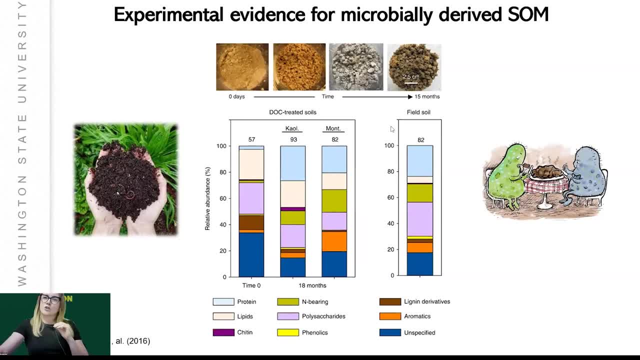 remarkably different number of compounds And you can see over here on the right hand side the field soil is remarkably similar. So this is just a soil that was taken out of a field, So nothing done to it at all, nothing added to it. 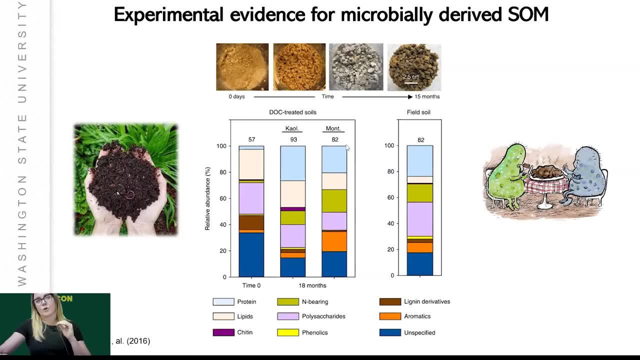 Can see that the field soil really starts to, or these soils start to closely resemble the field soil over time. So this is thought of to be direct experimental evidence that these microbes are actually building soil organic matter. And so what is the verdict? What does all this really mean? 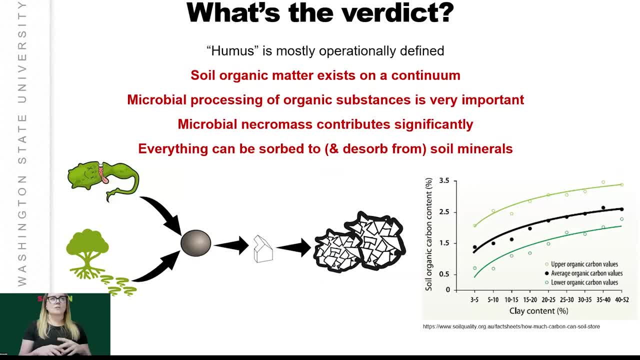 So essentially, this idea of humus, that was something that stuck around for a very long time and definitely became a bit of a buzzword in the agricultural community, as you can buy all sorts of humic substances to put on your soils. Humus is mostly operationally defined. 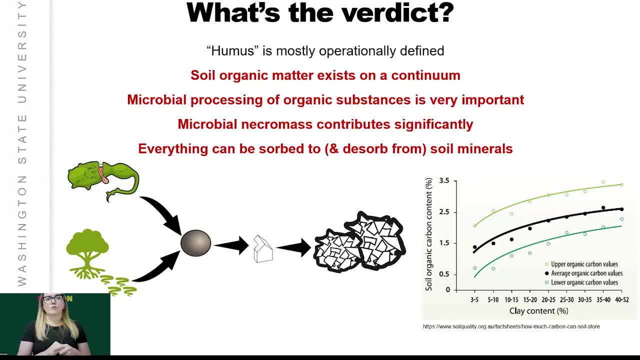 There is very little evidence that there is anything really that microbes can't degrade, But that soil organic matter does exist on that continuum And, as I said, things sorb to and desorb from soil minerals, And I'm gonna talk a bit more about aggregation here. 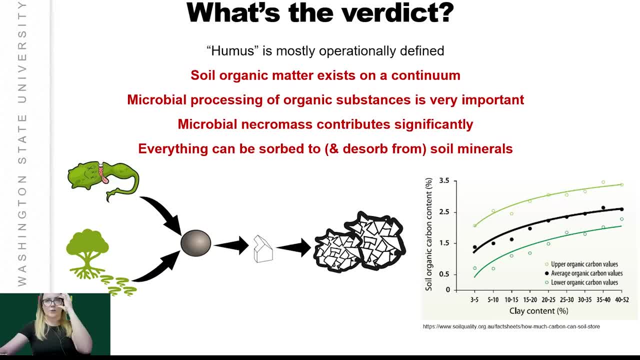 But that microbial net from us is a massive contributor to to soil organic matter And the stabilization of that plant material and microbial net promise is all related to that progressive sorption to minerals, to into micro aggregates, So small aggregates, that sort of soils. 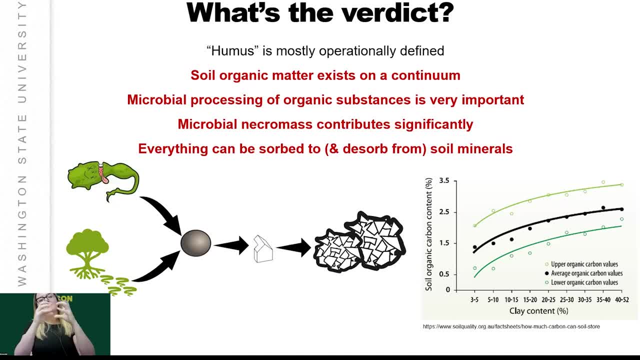 like forming, together with parts of organic matter, into larger macro aggregates. So, and this is sort of- I think, a bit more than that- of the basis behind, some of you may have heard of the fact that clay soils, or soils having more clay. 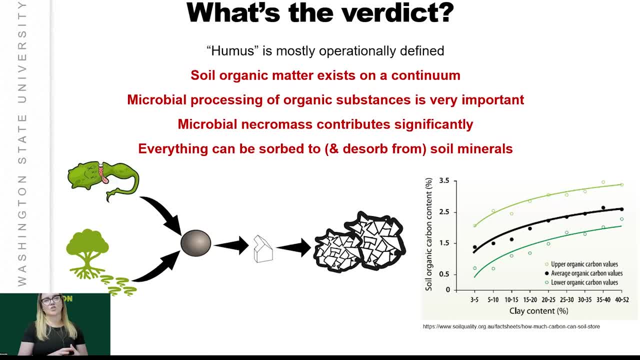 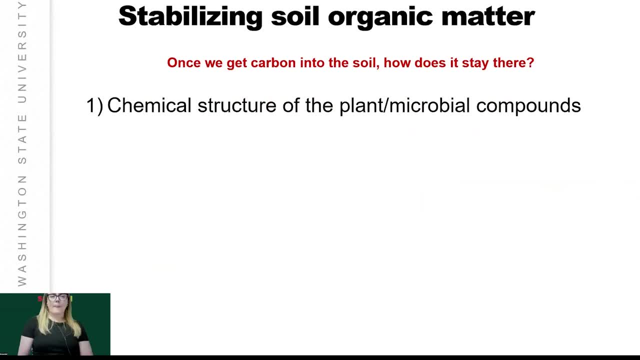 rather than sand, have a better capacity to store soil organic carbon. So once we get the carbon into the soil, how do we get it to stay there? So a lot of it has to do with the chemical structure of the plant and microbial compounds. 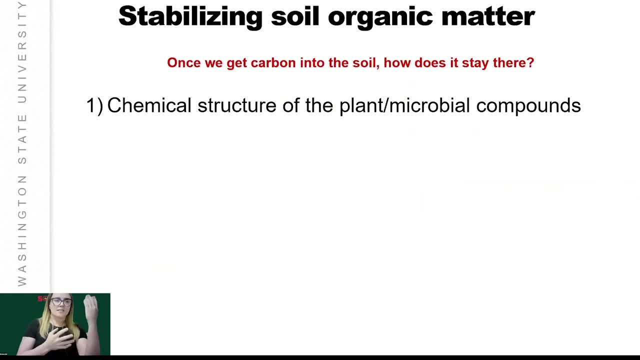 So I talked a little bit before about C to N ratios, the amount of carbon to nitrogen that plants have in it. Also, you have things like aromatic compounds that are parts of plants that are supposedly a little bit more resilient to chemical breakdown. So this is definitely a 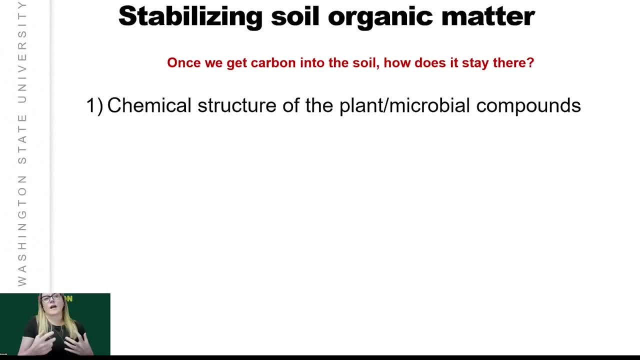 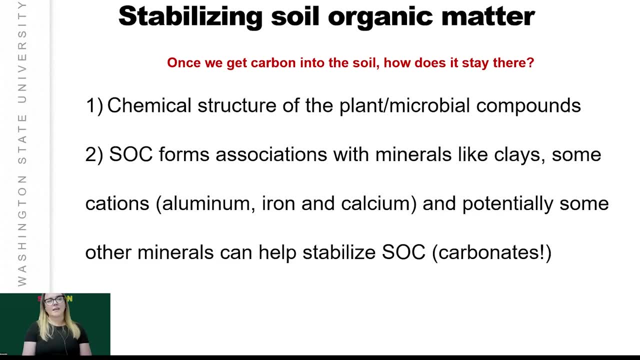 major component of whether or not carbon stays in soil and how long it stays in their form. But, most importantly, SOC needs to form association with minerals and clays, and it also does so with some cations as well, and some other minerals can help to stabilize SOC, like carbonates. I'm going to talk a little bit about that. 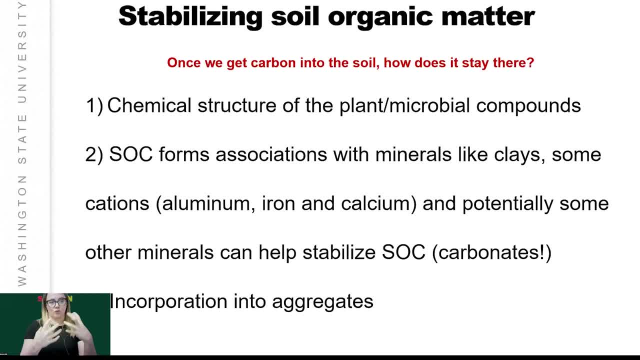 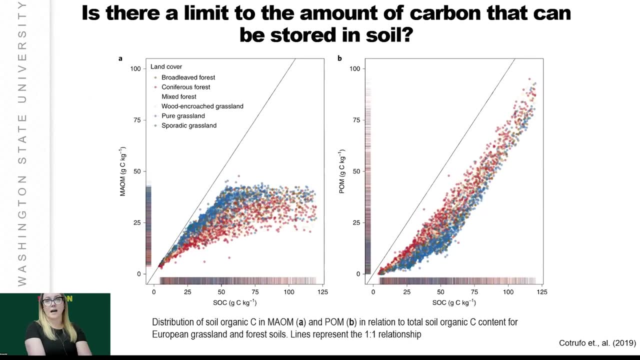 And again, we want to try to get that soil, organic carbon, to incorporate into aggregate structures, So larger and larger structures. So a lot of people have asked me: is there a limit to the amount of carbon that can be stored in soil? The answer is definitely, definitely yes. So this is a little bit more recent study from: 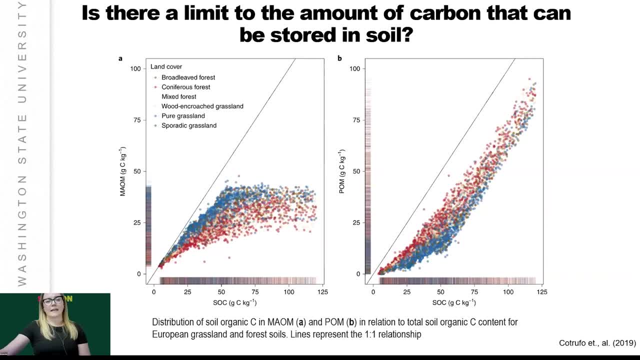 where they were looking at the distribution of soil organic carbon in MAOM, Mineral Associated Pools or particulate organic carbon. So in the soil science community we think about MAOM as kind of more that maybe heavier fraction, that more recalcitrant, so sticks around for longer fraction of carbon because of that. 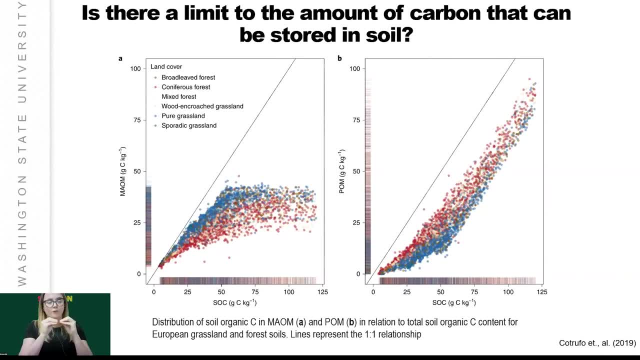 that absorption to minerals. It's protected somewhat from a decomposition. Then you have your POM, which is particular organic matter. Can be animal residues, can be mostly it's plant residues. You can kind of think of this as a little bit like the fluffy portion. 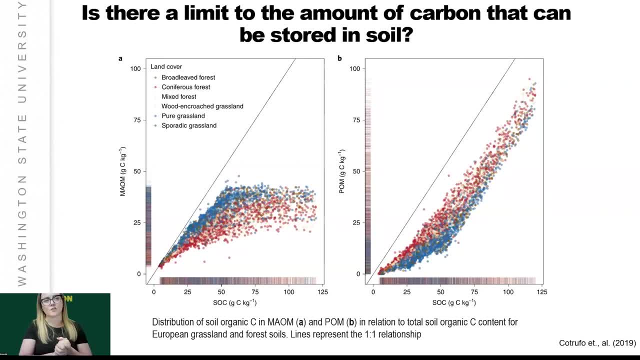 of soil organic matter, the lighter fraction of soil organic matter. So these guys did a study of all. these are all natural systems. none of these were agricultural systems. But you can see that in there's this kind of steep incline of the ground. 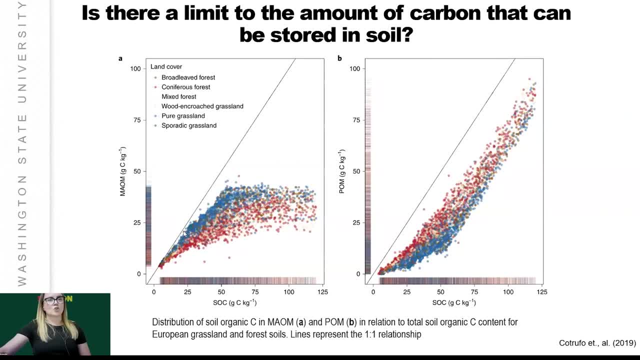 growth of soil organic carbon. in relation to how much mineral association is allowed, It gets to a certain point and once that point, once it's saturated, it tends to kind of balance off. So you don't kind of just get more and more and more SOC over time, forever and ever. It's basically. 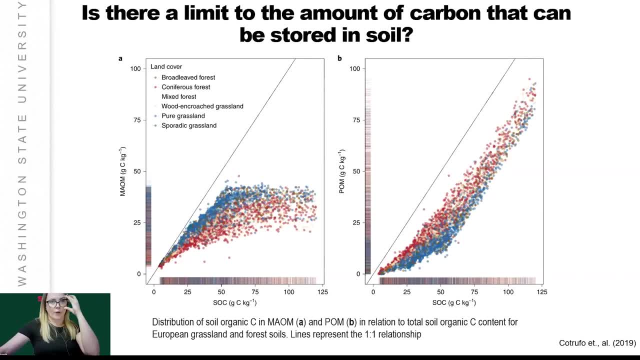 you know, it reaches a saturation point with the, with the mineral structure of the soil. but then, basically, what happens? it's not as if the soils don't ever accumulate any more carbon, but what they do is they continuously, progressively accumulate carbon in that particular organic matter fraction. Now why is that important? It's important because the particular organic 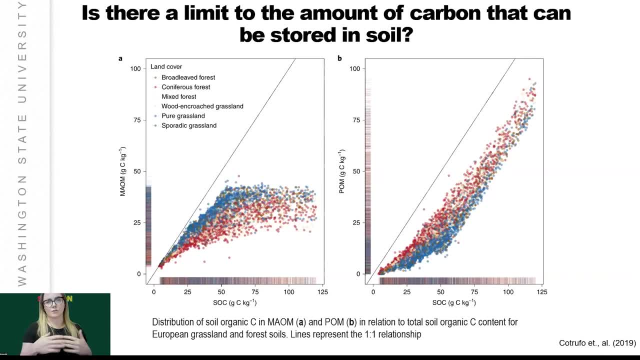 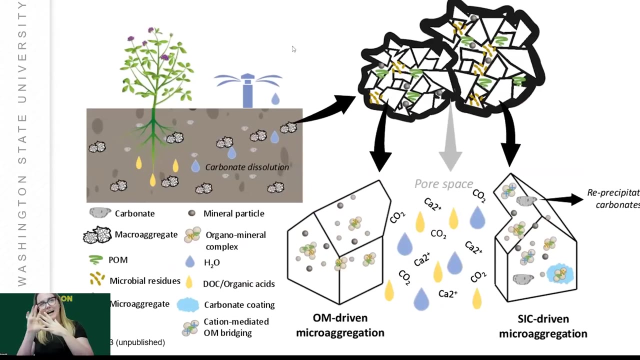 matter fraction is a fraction that can be more easily degraded. It is not. it's thought of as the faster cycling fraction, While ever soil organic matter, soil organic carbon, is not mineral associated. it is more susceptible to being lost from soil, So this is a little bit of a kind of aside. this is stuff that is very much new, I guess. 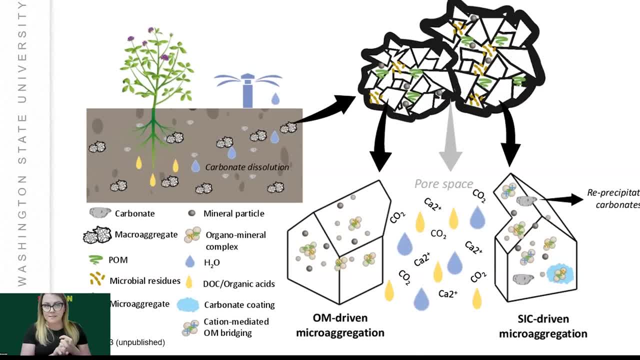 as far as the soil is concerned. So this is a little bit of a kind of aside. this is stuff that is very much new, I guess, as far as the soil is concerned. So this is a little bit of a kind of start to look a little bit more into arid systems and carbonate containing soils in particular. 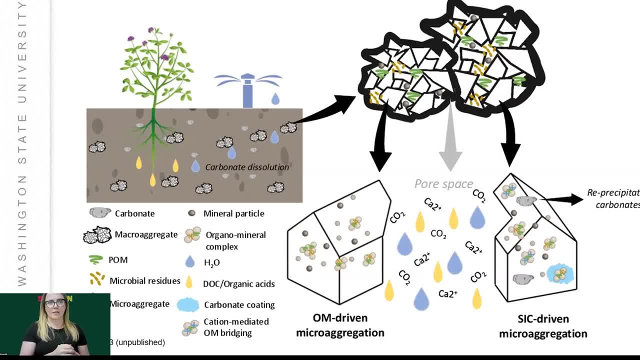 for their capacity to soil a soil organic carbon. I talked about clay as being the primary, primary mineral association that soil organic carbon has, but there are potentially other other abiotic, so non-biological, processes at play that could stabilize soil organic matter. So in carbonate containing soils, especially in agricultural systems, as we enter, as we introduce. 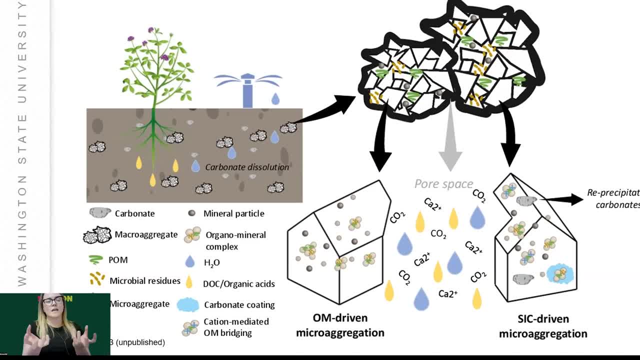 organic acids into the soil and we irrigate the soil, the natural carbonates that are in the soil can start to dissolve, Okay, so they go into solution and the products of that- that dissolving of the carbonates- move through the pore spaces in the soil and soil. organic carbon has been shown in 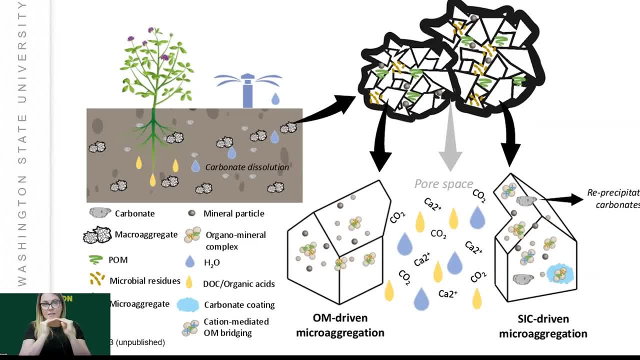 the literature to be a very important component of the soil. So this is a little bit of a kind of a kind of a very important point in the literature to make bombs with calcium cations, and that is another stabilization mechanism for soil. organic carbon that is not very well explored, But also 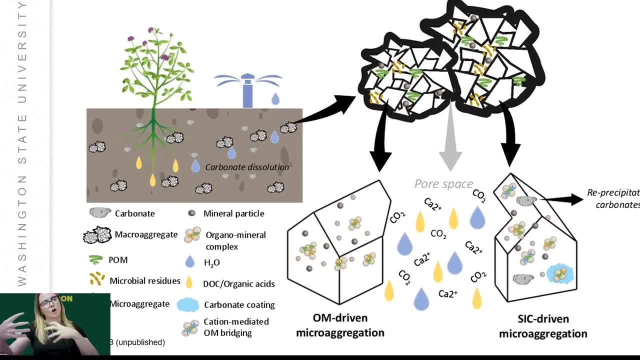 as those carbonates re-precipitate, so they will dissolve. but as we enter, as CO2 enters those core spaces, it will go back into solid form and soil organic matter can potentially get kind of stuck in these- uh, in this soil organic matter. So this is a very important point in the literature to make. 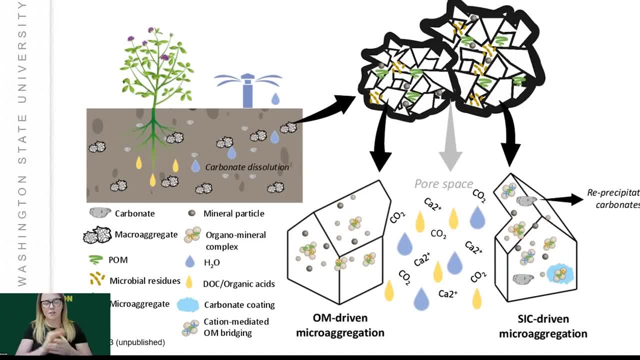 these carbonate. I call them cementations essentially. So there is a really uh, a whole kind of untapped area of soil organic matter stabilization uh that we're only just really starting to understand, and the majority part of that is because most uh of the research on soil organic 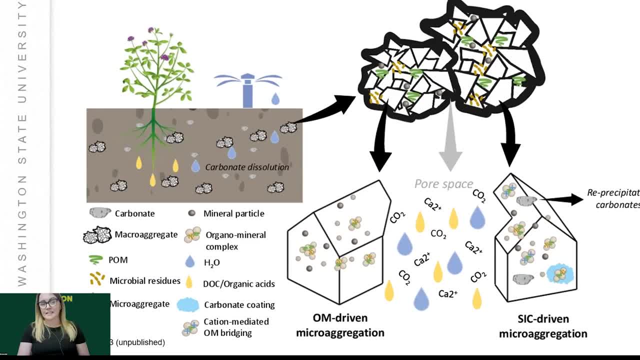 matter. accumulation, unsurprisingly, has been done in temperate systems, with very little attention being paid to systems that have a lot less carbonate and a lot less carbonate. So this is a very important point in the literature to make, but also the problem with soil organic matter. 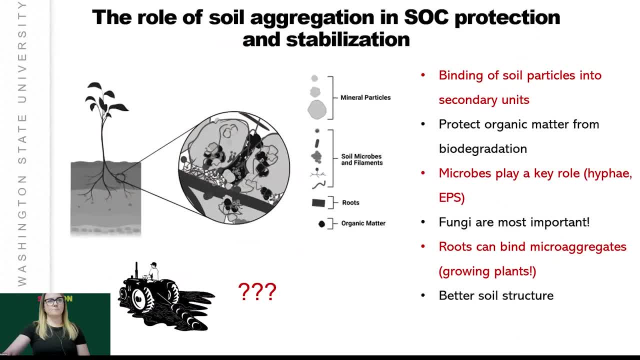 is that these are very important to understand these already existing systems Um that we are very vulnerable to this as it is. So it is important that we understand that there's a lot more carbon in the first place, soil, organic carbon in the first place, but that may have more soil. 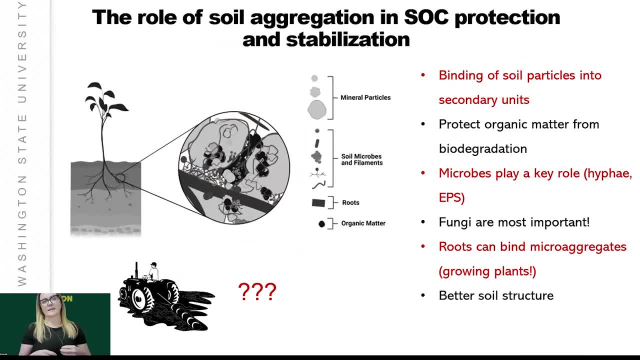 inorganic carbon. So I've talked a lot about, uh, the stabilization through mineral association. but what is soil aggregation and how does it help SOC be protected and stabilized? So, essentially, aggregates are these kind of secondary units. You get the minerals and then the minerals attached to. 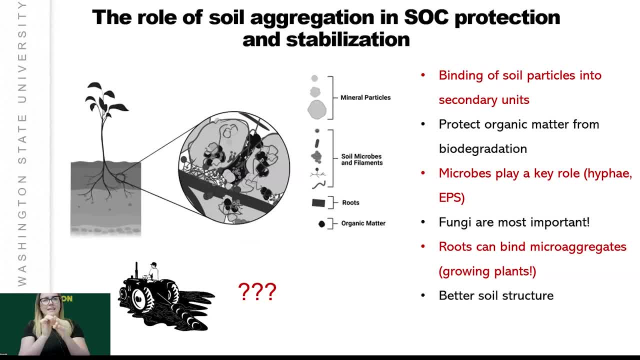 the minerals and you end up with these tiny little aggregate structures. It's very simple in the idea that they just protect organic matter from being accessible from microbes- If you think about the soil matrix as kind of like this environment where they can all kind of move around and 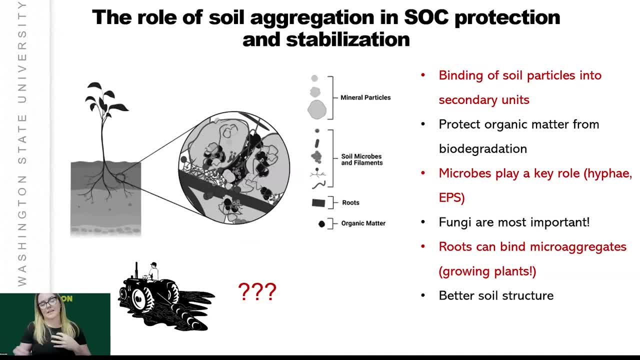 everybody's trying to access nutrients. they're just being protected a little more inside aggregates. But microbes also play a large role in making these aggregate structures, particularly fungi, as they have structures called hyphae and they secrete these extra polymeric substances which is kind of like this blue that helps aggregates kind of stay together. 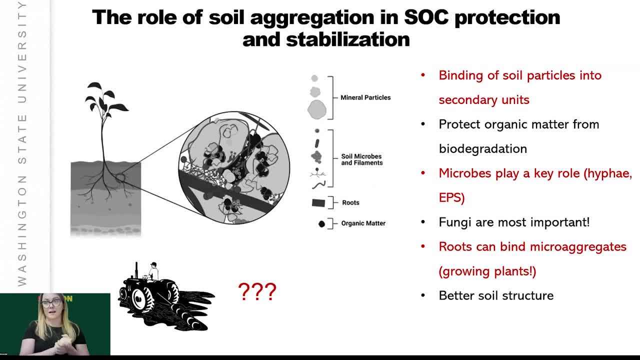 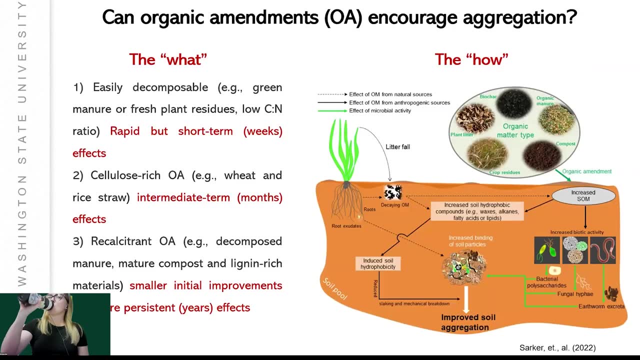 Roots. plant roots also bind microaggregates into macroaggregate structures, So growing plants and always going to be a thumbs up for a soil aggregation. So a part of my research at CSA and I was looking at whether organic amendments can encourage soil organic carbon storage in soils in Washington. It's not a very simple answer. 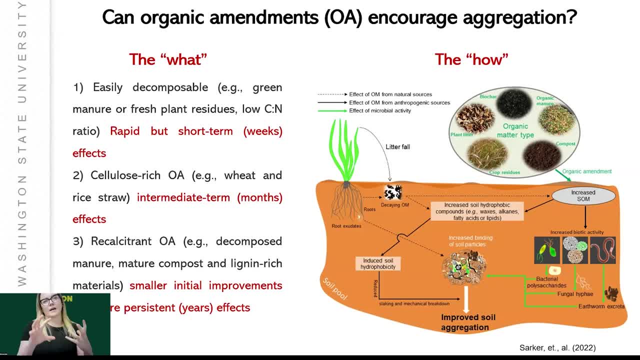 I have to say. but I'm going to talk a little bit about how organic amendments might actually encourage aggregation in soil, And then you can start to kind of take your mind around how that might help with carbon storage. So I mentioned before that it. 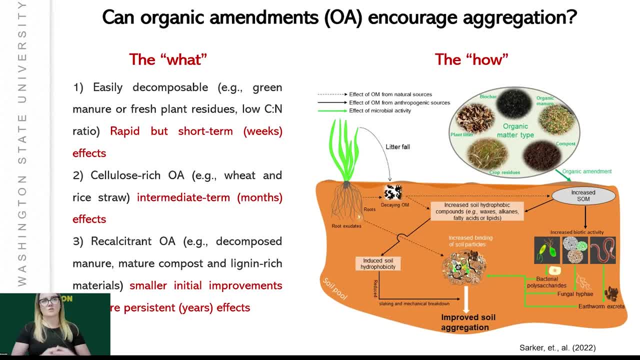 is important to understand what kind of residues we're putting into our soil. So things that are more easily decomposable, something that has a low carbon to nitrogen ratio, might have a rapid effect on soil, organic carbon and on aggregation. So I'm going to talk a little bit about that. 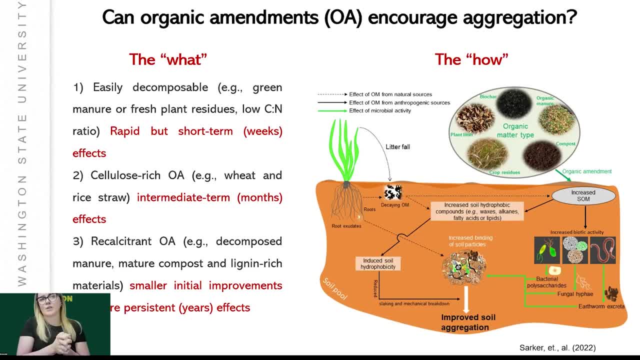 So a part of my research at CSA and I was looking at what kind of residues we're putting into our soil, So things that are only decomposable. something that has a low carbon to nitrogen ratio might have a rapid effect on soil, organic carbon and on aggregation in the term of weeks, But it can be pretty short term. microbes can tend to maybe eat up those compounds a little bit faster. 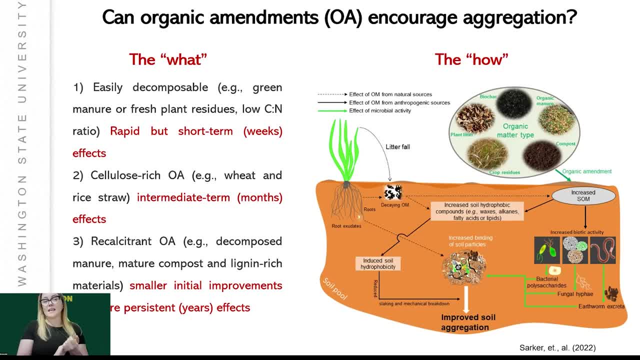 Then organic amendments that are a little more cellulose rich, like, if you're thinking about straw, mulch, rice straw- that could be something that might have an intermediate term effect over a period of months. But again, a little bit better than that, that kind of rapid short term effect, but still not not as very effective. So that's really important. And so the first thing I'm going to look at here is what kind of organic amendments and the two things are best for digesting our soil, For example. well, a few things like 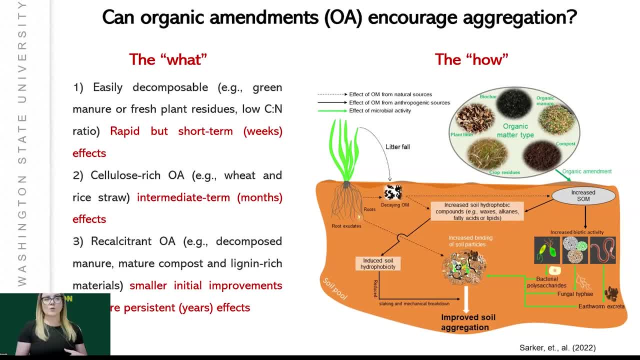 as stable as some other compounds, like composted manure and decomposed manure and things that are very lignin rich, which might make initial improvements pretty small. so it's important to think about that when you're when you're trying to assess whether or not your organic 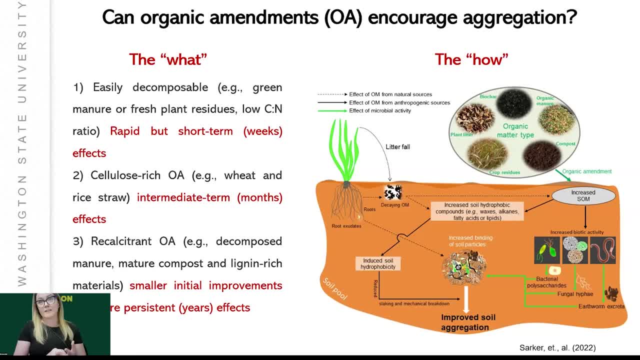 amendment has actually done anything. you may not be seeing it in the short term, but these effects with more recalcitrant, more difficult to kind of decompose, tend to be more persistent over years. so organic amendments encourage aggregation by being an exogenic source, so coming from the outside, 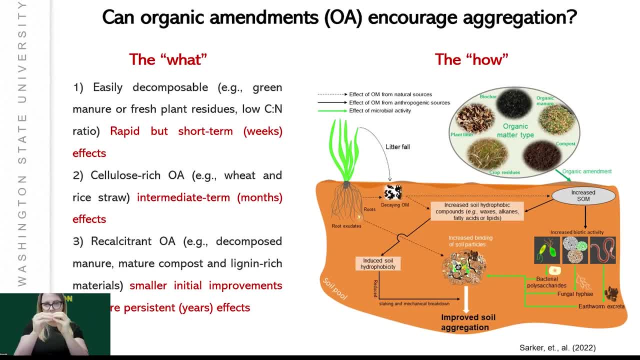 and they just increase soil organic matter in that, in that exact moment. but it's not so much the fact that we put organic matter in the soil that we can say, oh, we're just storing more carbon. it's all of those follow-on processes that happen afterwards where we're seeing the benefits of organic amendments. 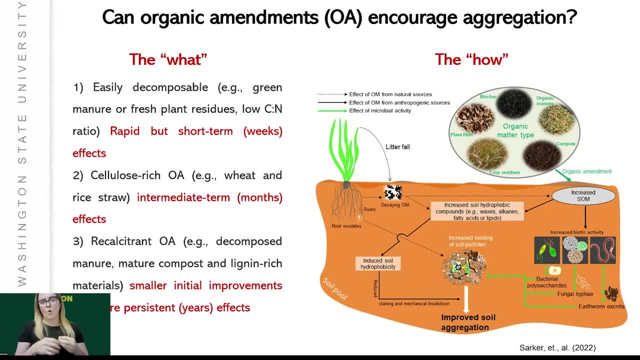 and that is primarily in that more aggregation is being induced with organic amendments. that has to do with the increased biotic activity- you're giving the microbes more food to eat. but also there's different kind of compounds that are being introduced with exogenic sources, like manures and composts that increase the hydrophobicity of soil, which essentially 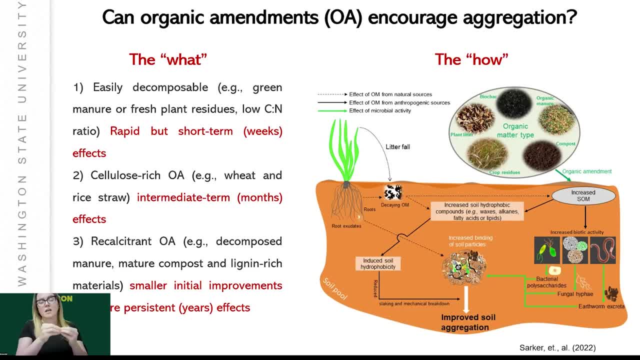 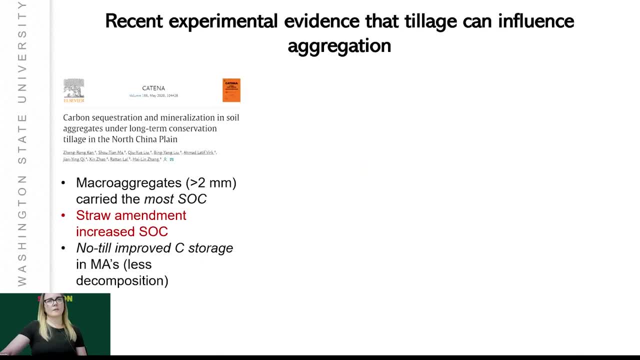 allows whatever aggregate structures are there to to not flake or or to be broken down mechanically, and all you need to do is go on very quickly to google scholar. i literally picked probably just four of the most uh, uh recent um articles that we're talking about organic amendments, um, and how they might increase aggregation and uh, increase therefore. 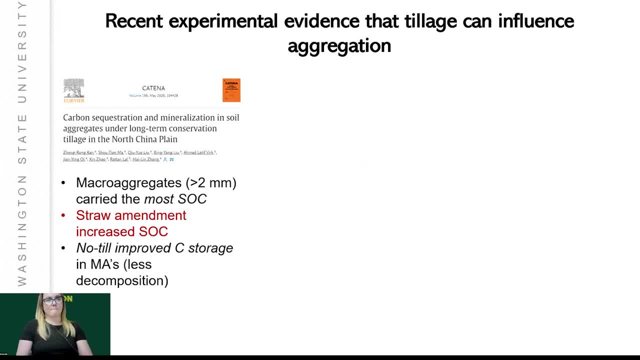 soil organic carbon storage, so um, macro aggregates, so those larger aggregate structures carried the most soc in this particular um study and that straw amendment increased soc. you remember before i talked about straw residues having a more kind of intermediate effect on soil organic carbon storage, soil aggregation, And we're going to talk a little bit about no-till because this is a little bit. 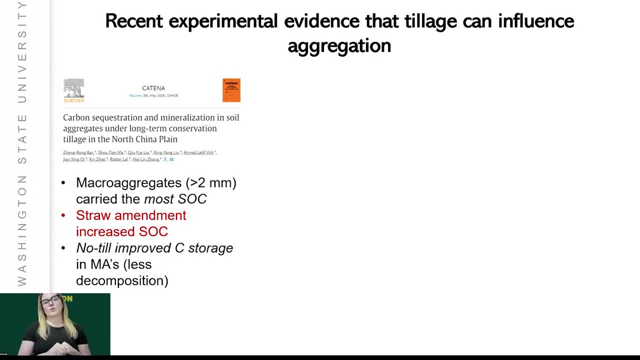 about management: No-till improves sea storage in those macro-aggregates and that was through the process of reducing the amount of decomposition that was happening from a microbial standpoint. Another one about tillage: carbon and nitrogen was higher in aggregates under a no-till system. 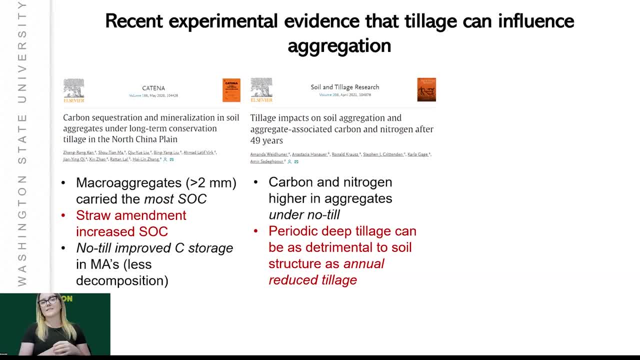 I found this really interesting: that periodic deep tillage could be just as detrimental to soil structure as annual reduced tillage. So it's perhaps also not necessarily just the tilling itself, but it can be the well. we do know that it is the extent to which that tillage is occurring. 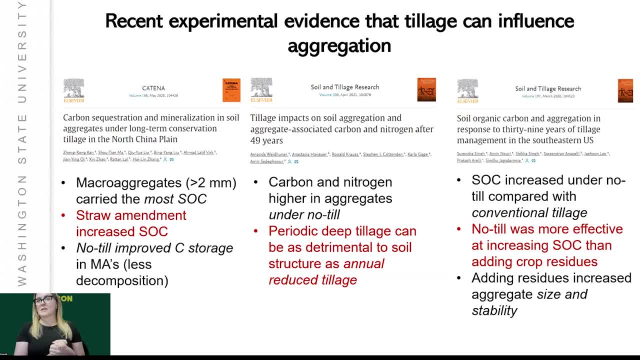 and how often, And in this particular study, over quite a long time. in the southeastern US, they found that SOC was increased under no-till compared with conventional tillage. This is not an unusual thing to find in a lot of these studies, but I found in particular, 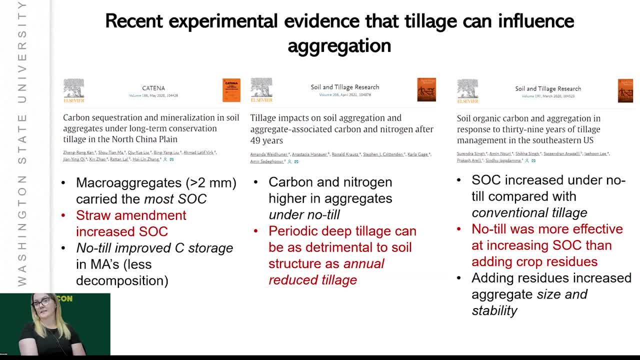 interesting that no-till was more effective at increasing SOC than adding crop residues. So I think that Randy kind of touched on this a little bit before about somebody asked about annual systems and their ability to store SOC. It's absolutely, it's absolutely, it's absolutely. 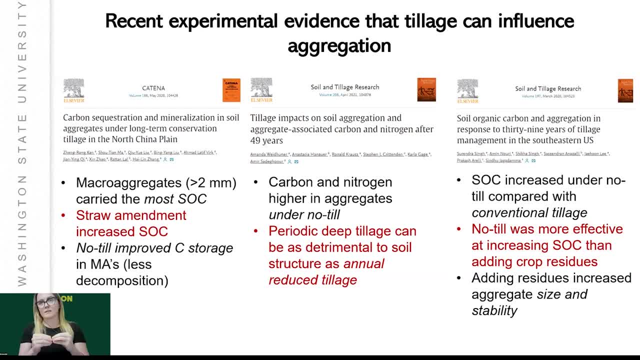 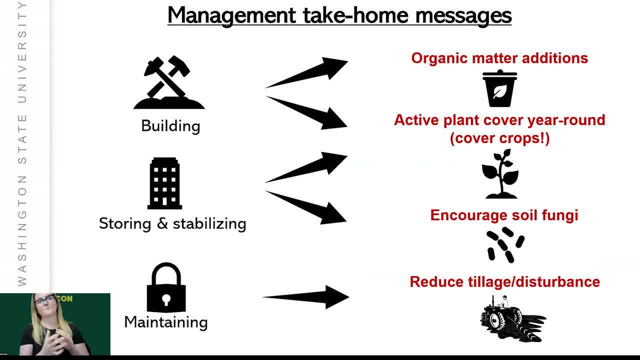 the focus on keeping what is already in the soil. that is really, really important, in addition to adding crop residues, but protecting SOC. So this is my wrap-up slide. So management take-home messages. So, in building soil, organic carbon, what can we do? Let's take advantage of exogenic. 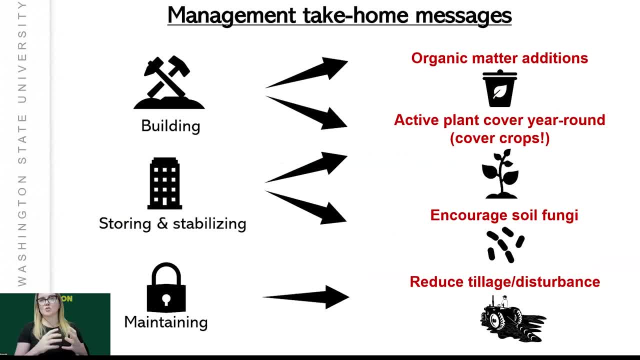 sources- organic matter additions- but paying attention to what those organic matter additions look like And having active plant cover over time. cover cropping, grassland restoration, as Randy talked about. that is going to help us not only to build more but also to store more as those root. 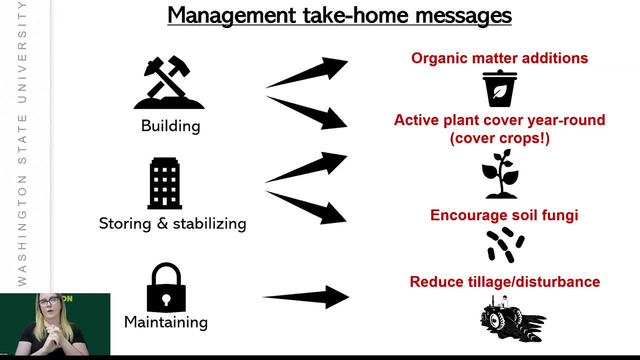 structures will help to keep those aggregates together. We want to encourage soil fungi. I would encourage you to have a look at how you can encourage soil fungi over bacterial communities. It has a lot to do with, again, the C to N ratio of things that you're putting into the soil and 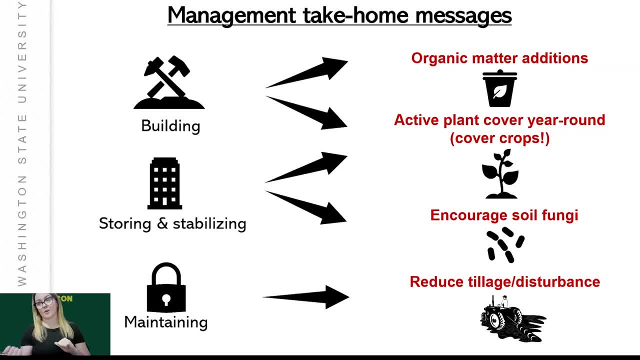 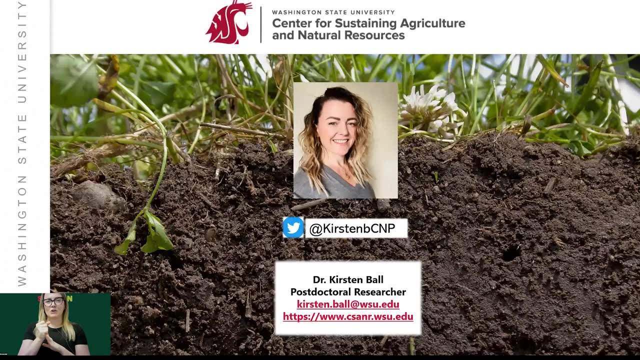 things like fertilization, which can increase soil bacterial versus fungal communities, And if you want to keep it in there, you need to reduce tillage and disturbance over time, And I think we've heard a lot about that, And that's all I have time for today. I think I've gone over even a little bit. 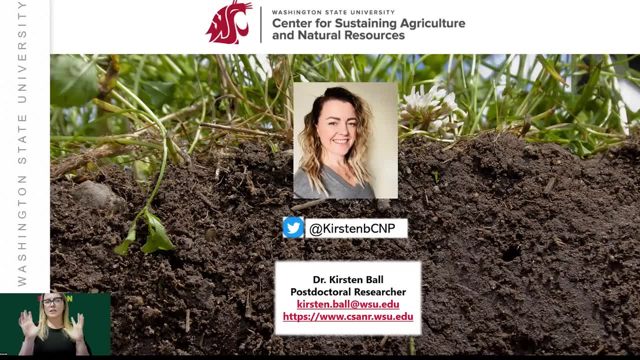 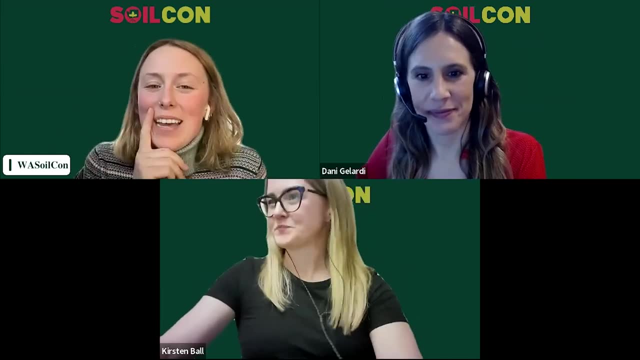 but if you would like to follow me on Twitter, I would love to see what everybody is doing, And thank you very much for having me today. Hey, Kirsten, I'll go ahead and ask some questions that we got from the chat. We have one: what does soil? fungi populations have on sequestering carbon for humus formations. Any thoughts on that? Okay, well, first of all I would have to say Okay. Let me address how soil fungi can be really helpful at helping us sequester soil organic carbon. 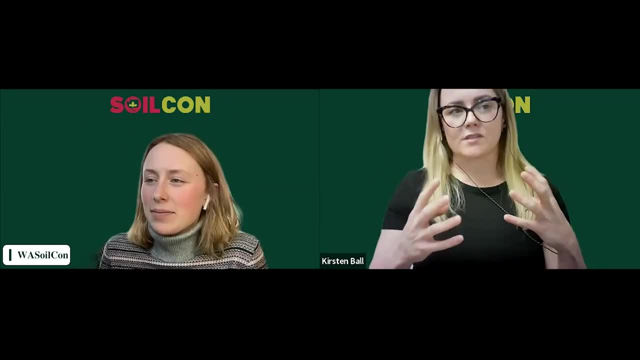 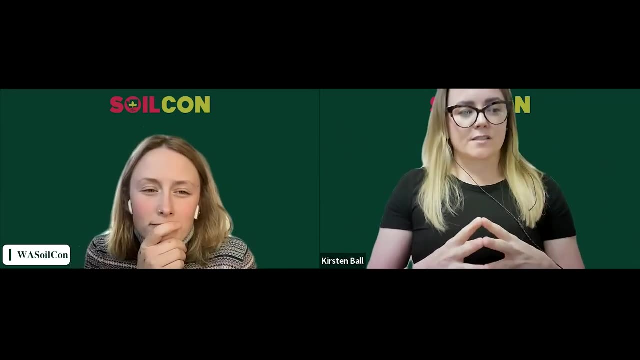 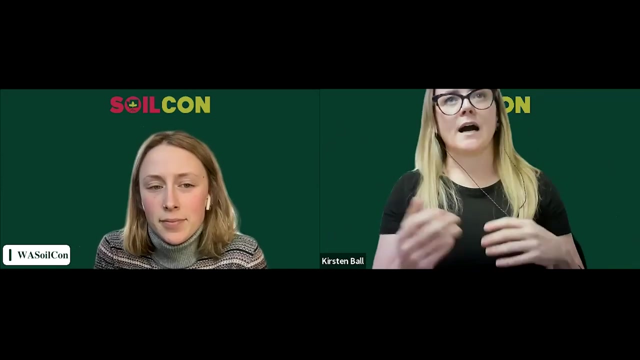 But remembering that I talked about humus as one of those kind of things that we thought existed but we found out that it really didn't. Essentially, there is only really one, let's say storage of carbon, that could be argued to be of thousands. 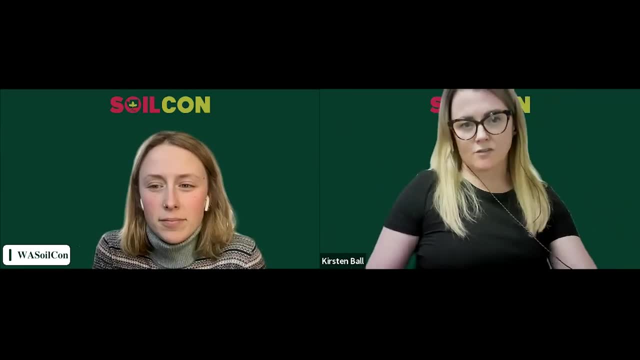 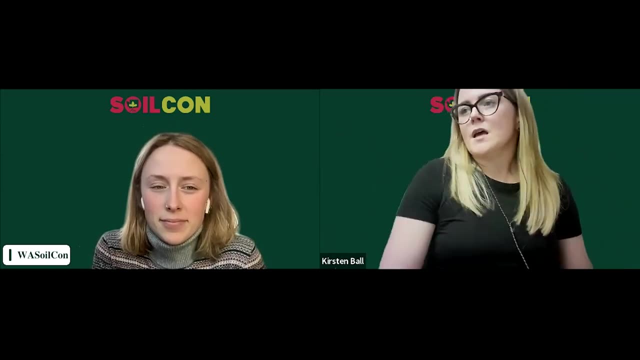 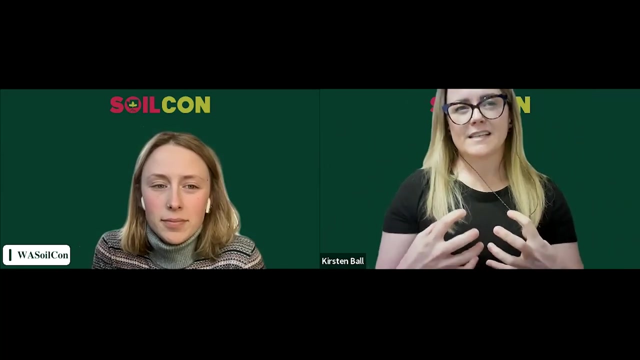 of years and that is carbon of pyrogenic sources, so essentially after burning and things like biochar for example. But soil fungi actually help us to build soil organic carbon, insofar as they're almost kind of like the trudgers. of the soil community. They tend to kind of cycle soil organic carbon a little more slowly And also there's There is some evidence that they have a better time at breaking down more kind of higher C to N ratio organic matter than bacterial communities. 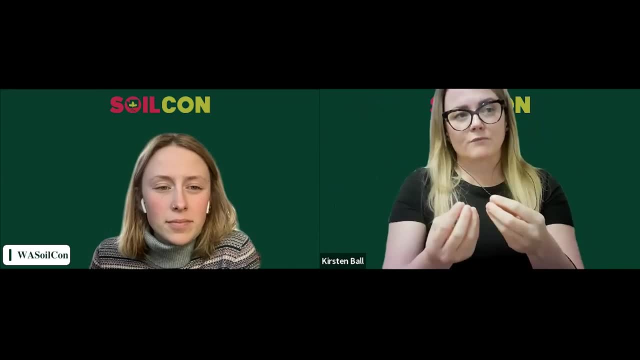 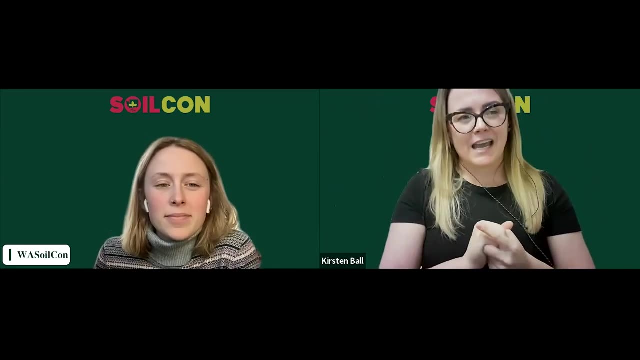 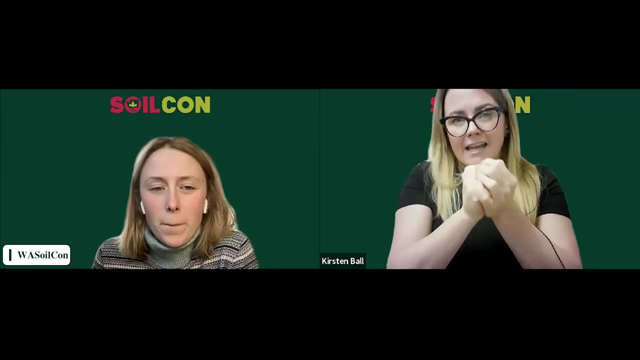 But one of the most important things is really some of those substances and the components of their fungal anatomy- I could say that help to pull soil particles into aggregates. So, for example, the C-cells are a really good example of how they're helping to build organic structures. 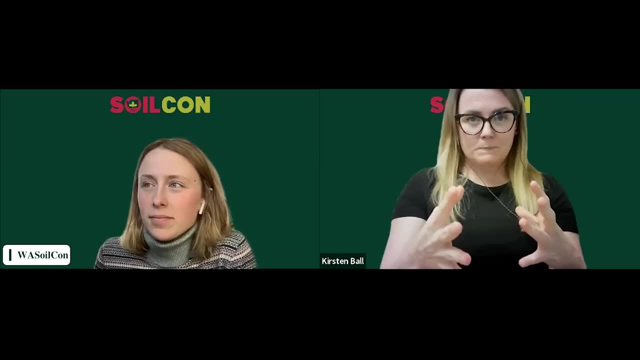 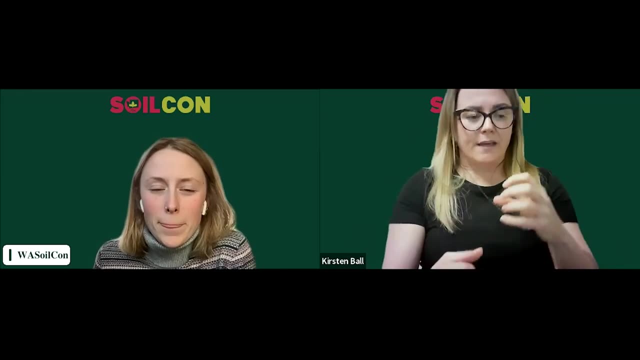 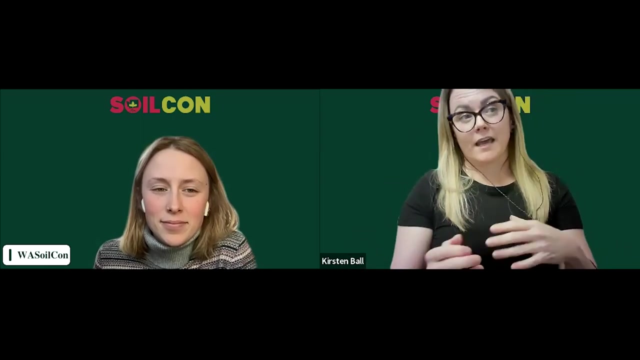 and help whatever carbon that is in the soil to stay in there. So I wouldn't necessarily say that they're building humic structures. I would say that they're helping to cycle soil organic carbon in a way that is a little bit kind of more slow as you go. 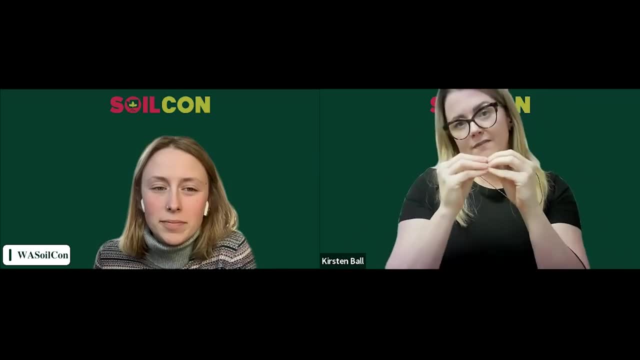 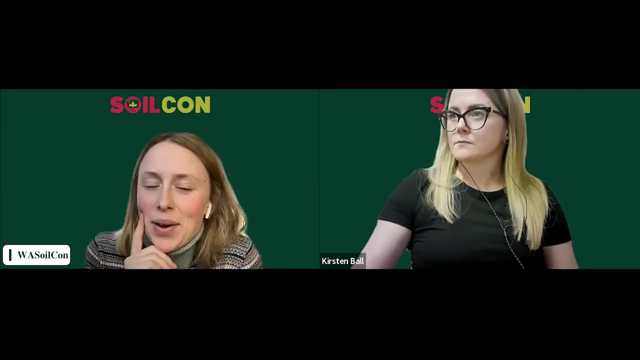 maybe a little more carbon use efficient than some bacterial communities, but they do have a little bit of a protection, So they kind of have a bit of a dual role, Gotcha, Okay, Thanks for clarifying on that. I know we're at time now, but I do have one question that I want to ask you. 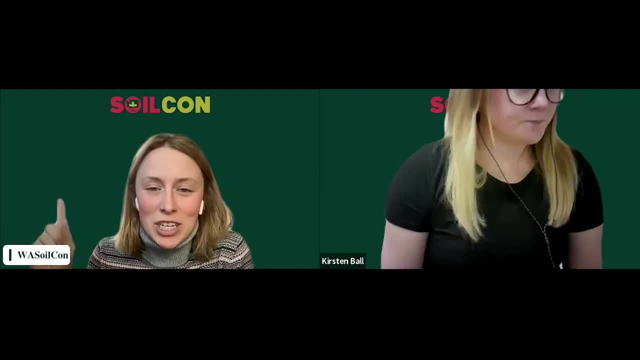 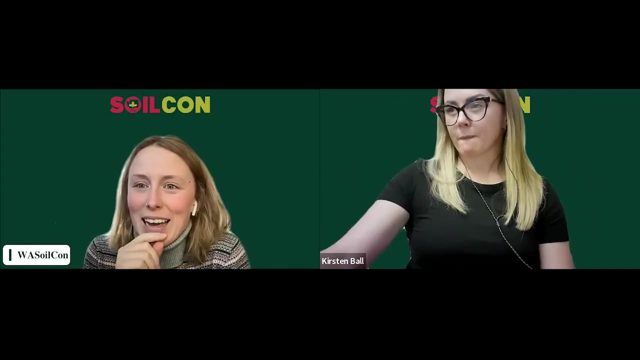 And. But before I do that, I want to encourage everyone to go to the Engage tab. answer that one question: survey on the quality of this talk. We'd appreciate that a lot. But the one final question and maybe yeah, in just like two minutes. 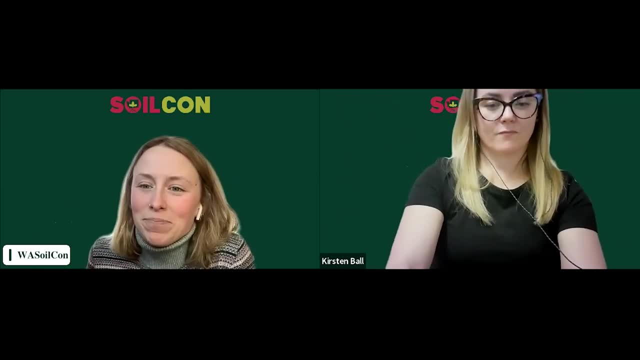 you and Randy both talked about The long-term impact of climate change on the environment, So what are some of the things that you would like to talk about? What are some of the things that you would like to talk about? What are some of the things that you would like to talk about? 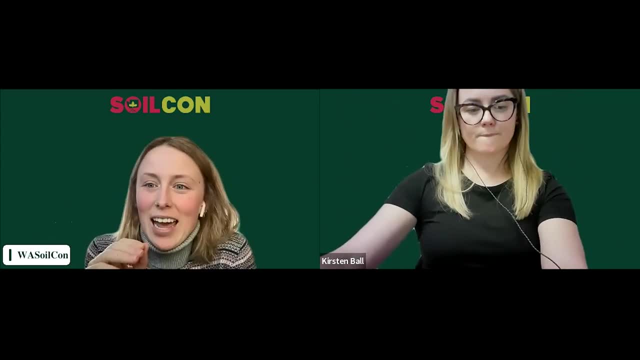 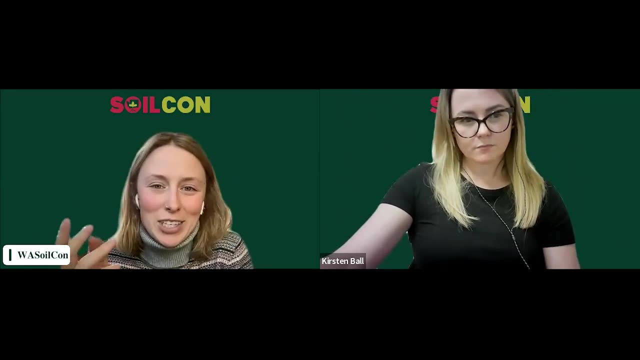 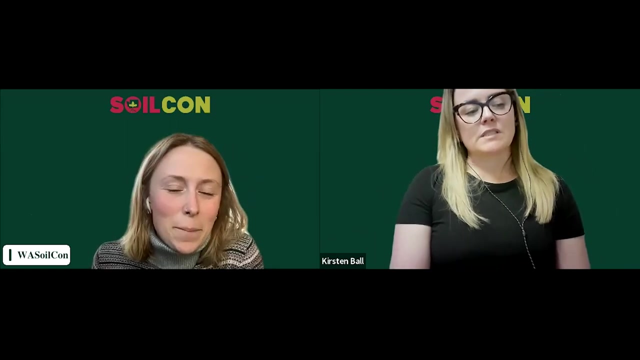 The limitations of soils under ag production and the ability to sequester carbon. Can you say more about the role that soils do or don't play in climate change mitigation? This is such a huge topic. Yeah, Yeah, I guess I would say that maybe it's a double-edged sword. 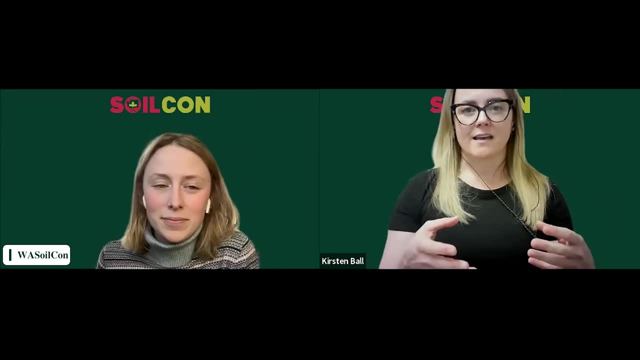 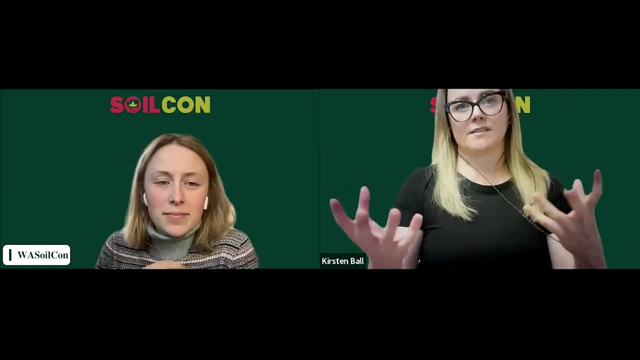 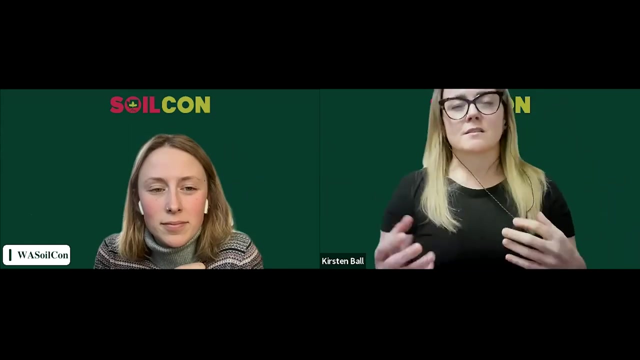 because, fortunately, soils have come into focus as a way that we can definitely sequester more carbon in soil. I mean, there's There's more carbon in soils than there is in the terrestrial environment and the atmosphere put together. But it would be a little bit amiss to say that soils are our solution.